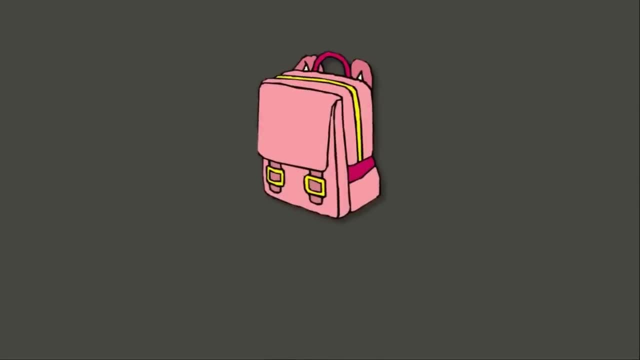 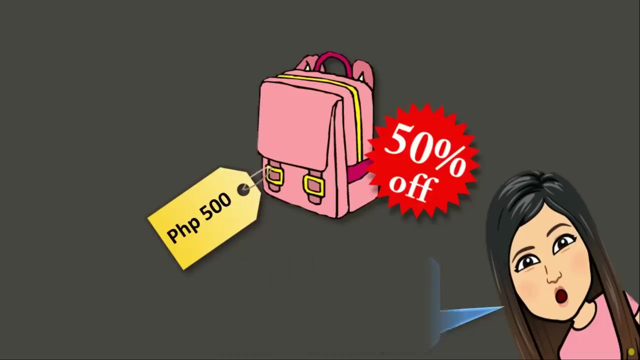 Let's say I am selling a bag which costs 500 pesos, But I decided to put it on sale with 50% off. Now how much is the discount? To get the discount we need to get the 50% of 500 pesos. 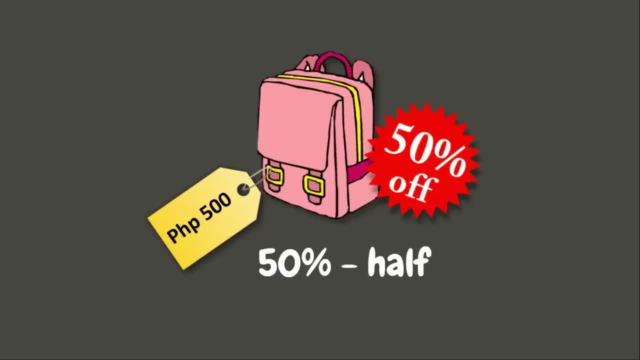 As we all know, 50% means half. This means that we need to get half of 500 pesos. Do you know what is 50% or half of 500 pesos? Wow, great job, You are right, It is 250 pesos. 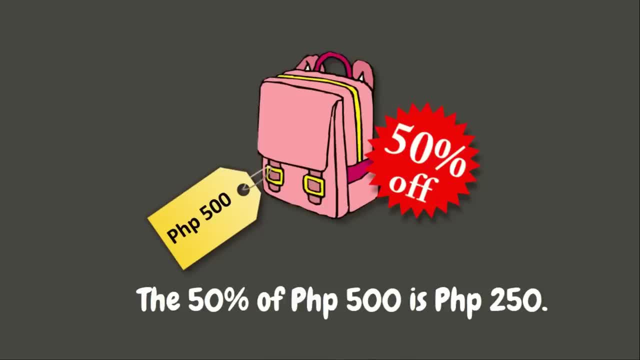 This means that the 50% off- 500 pesos- is 250 pesos. Now, in this given statement, this 50% is only 50.5.. This means that the 50% off is 250.5.. Now, in this given statement, this 50% is still only 500 pesos. 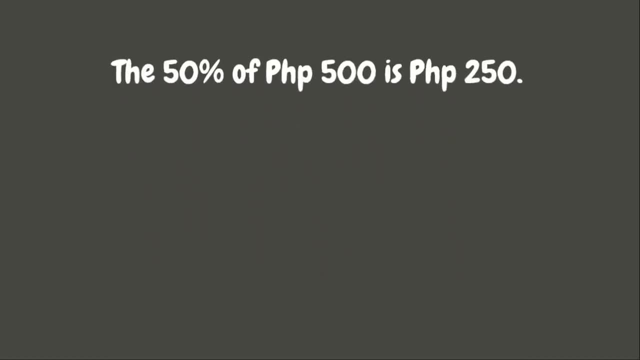 For example, let's try 5 times to find the percentage rate and base in a given problem. this 50% will cost 500 pesos. depending on how much this cost, 50% is the rate. Rate is also called percent, which has percent sign. 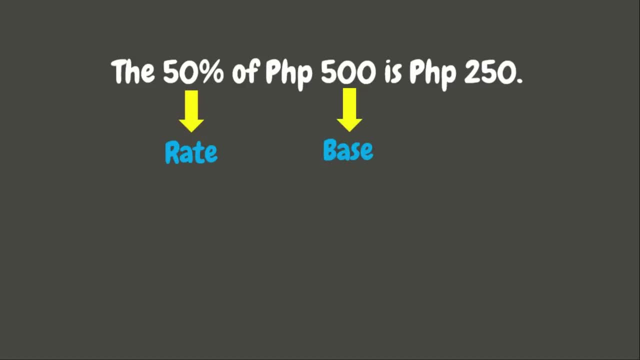 While 500 pesos is the base. The base is the entire or original amount which usually comes after the word of. And finally we have the percentage. 250 is the percentage. Percentage is the part or portion of the base which usually beside the word is. 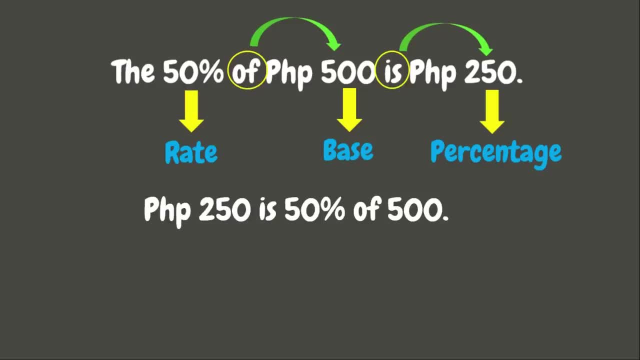 This statement can also be written as: 250 pesos is 50% of 500.. To identify the rate, base and percentage, let's take a look. If the number is beside the word is that is the percentage. While 50% has percent sign, that means that is the rate. 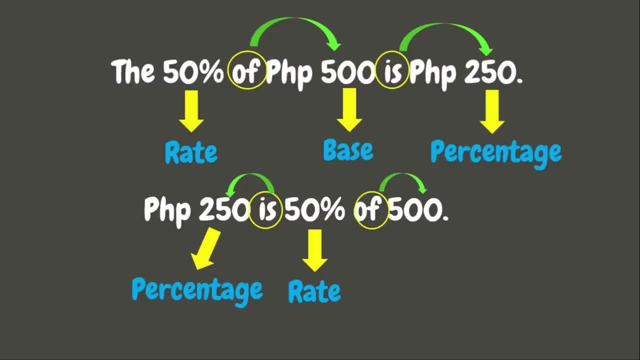 And 500 comes after the word of. That means that is the base. Very good Now did you know that the word of also represent multiplication, while the word is represent equal symbol. This means that rate times base equals percentage. That gives us: 50% times 500 pesos equals 250 pesos. 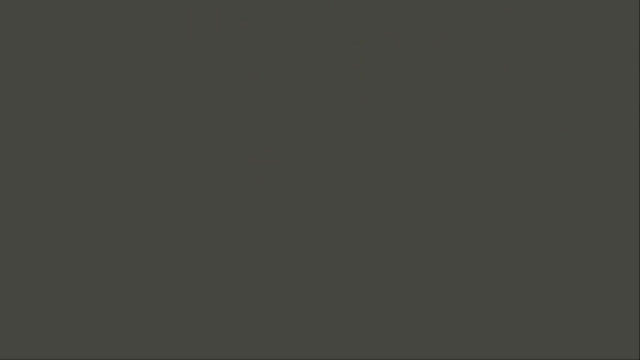 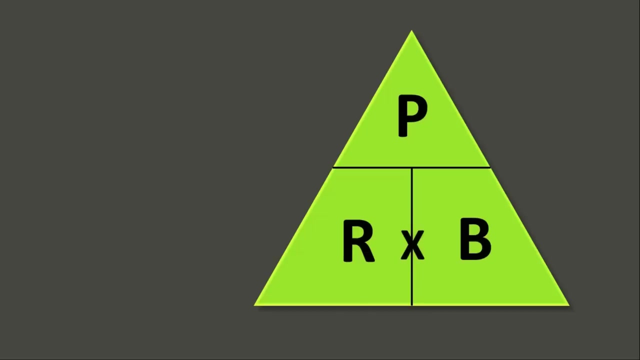 Now for us to get the rate, base and percentage in a problem. let us use the following formulas: To get the percentage, we need to multiply the rate and the base. That gives us the formula P equals R times B. Now to get the rate. 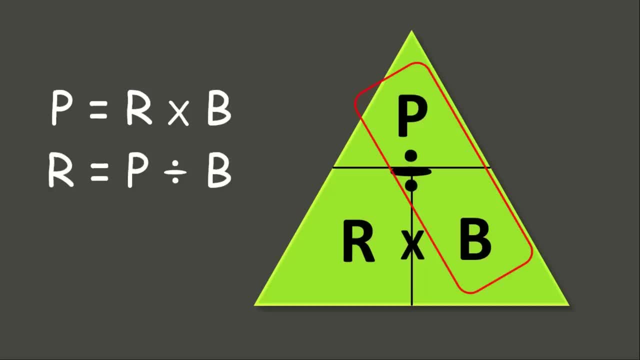 we need to divide the percentage by the base, And the formula is: R equals P divided by B. And lastly, to get the base, let us divide percentage by the rate. So our formula is B equals P divided by R. For us to easily remember the formulas, 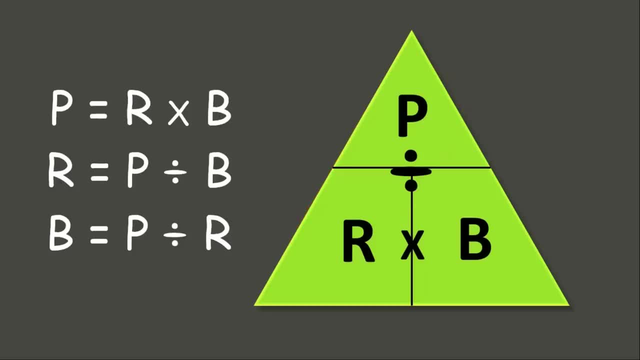 we can use this triangle If we are only looking for percentage. you may cover by your hand the letter P, which gives us R times B. If the missing term is the rate, simply cover letter R. That leaves us P divided by B. 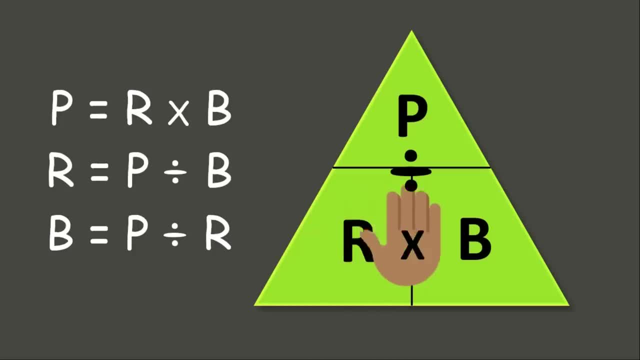 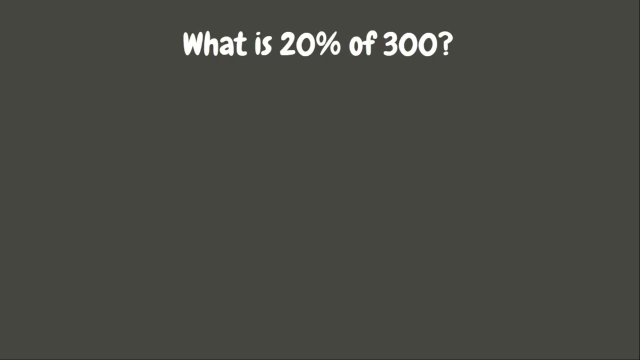 And lastly, for the base, the formula is P divided by R. Wonderful, Now you are ready to solve some problems. Let's try our first example. What is 20% of 300?? The first thing that we need to do. 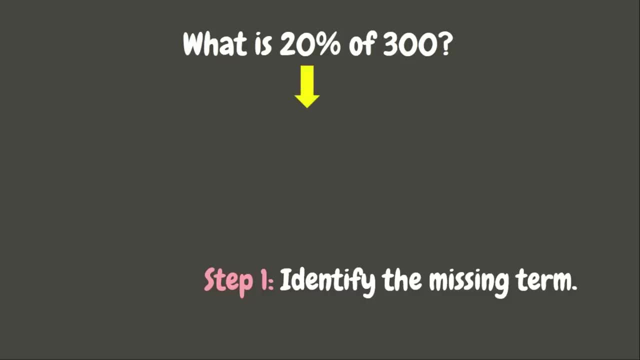 is to identify the missing term. We all know that if the value or the number has percent sign, that is the rate And the number which comes after the word of is the base. That means the missing term is the percentage which is beside the word is. 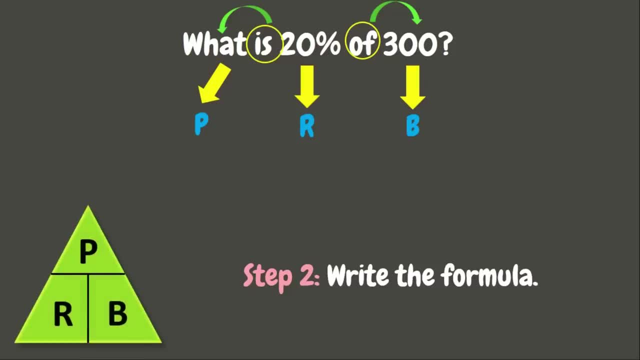 Now let us write the formula. Let's use our triangle To get percentage. we will multiply rate to the base. P equals R times B, 20% times 300.. The next step is to convert or change the rate or the percent into decimal. 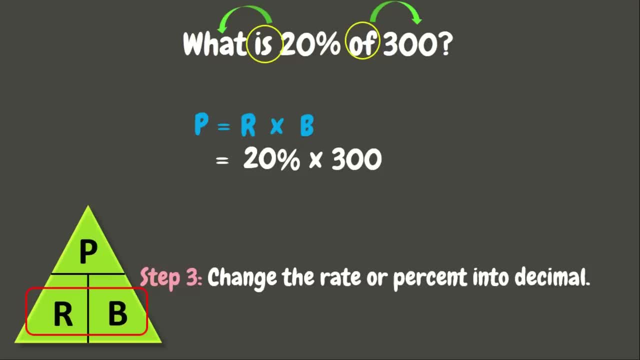 To change the percent into decimal. let's change percent sign into a decimal point. There you go Now. let us move the decimal point two times to the left: 1, 2.. There you go Now. 20% is now 0.20.. 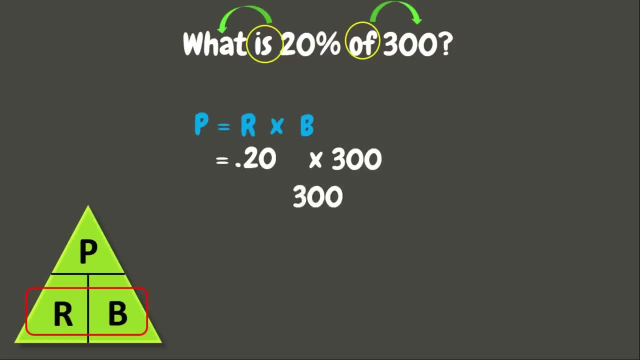 Now you are ready to multiply 300 times 0.20.. 0 times 300 is 0.. 2 times 300 is 600.. Now, let's add That gives us 6,000.. Now, since we have two decimal places here, 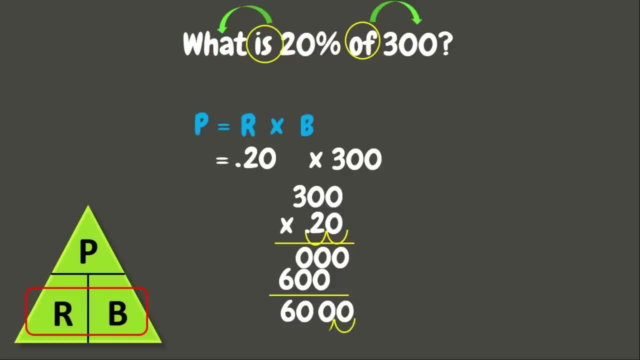 let us move the decimal point two times to the left. There Now, our final answer is 60. Therefore, 20% of 300 is 60.. Great job, Let's try another one. What percent of 24 is 12?? 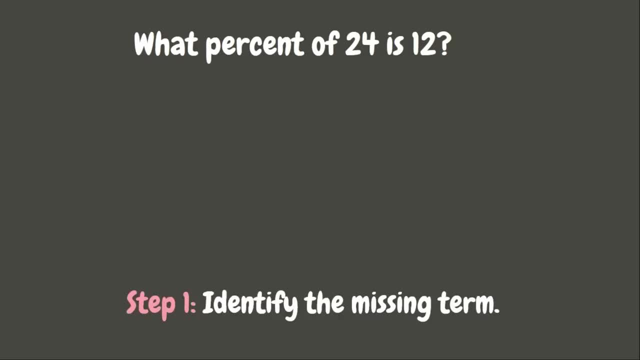 Again, let's identify first the missing verb. Since 24 comes after the word of, that is our base, And 12,, which comes after or beside the word is, is our percentage. And obviously the missing here is the percent or the rate. 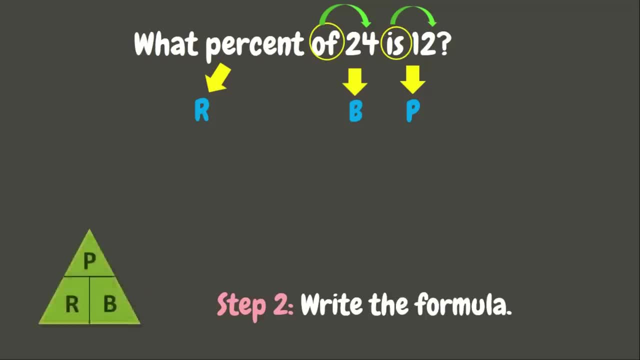 Now let's try. the formula r is equals p over b, or p divided by b. That means to get the rate we need to divide 12 by 24.. Now let's divide it: 12 divided by 24.. Since we cannot divide 12 by 24,. 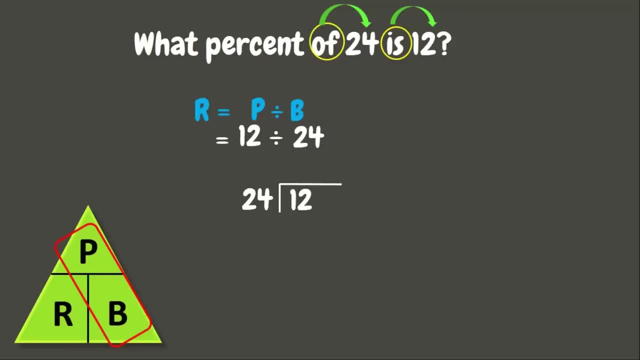 let's add 0.0.. There Now we have 120 divided by 24.. Let's put first the decimal point, a line from the decimal point, in the dividend. Now, 120 divided by 24 is 5.. 5 times 24 is 120. 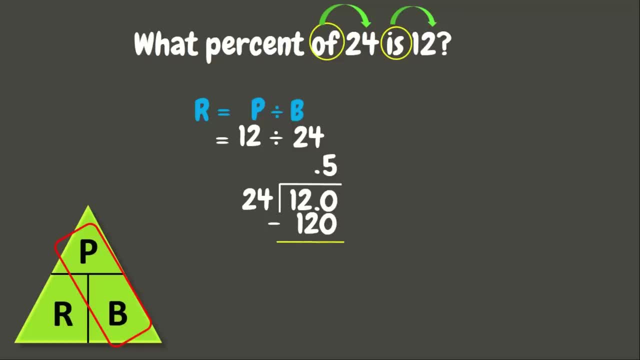 120 minus 120 is 0.. Now to get the percent, or the rate, we need to change the decimal to percent. Here, to change decimal to percent, we are going to move the decimal point 2 times to the right. 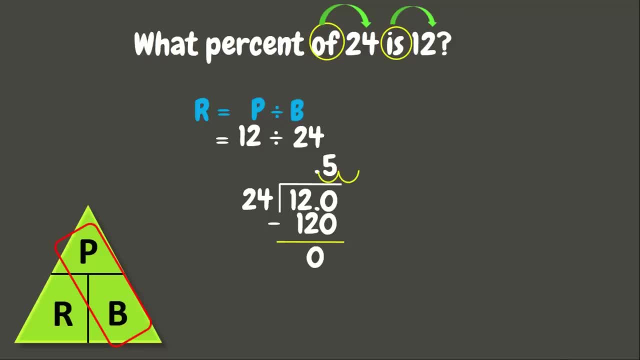 1, 2.. Since there is a missing place value, let's put 0.. Now let us change the decimal point to percent sign. Now our answer is 50%. This means that 50% of 24 is 12.. 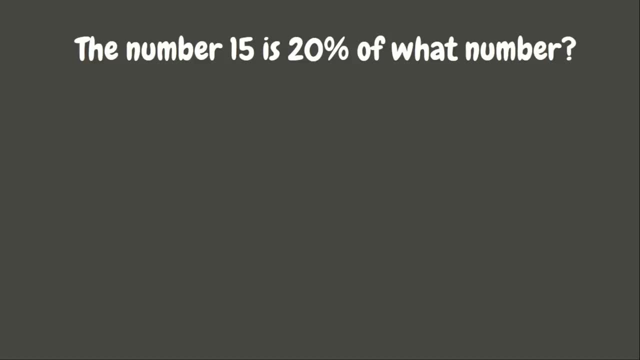 Wonderful. Alright, we have another one right here. Again, let's identify the missing term. Again, we all know that the one which has percent sign is the rate, While the number beside the word is is the percentage And the value or the term. 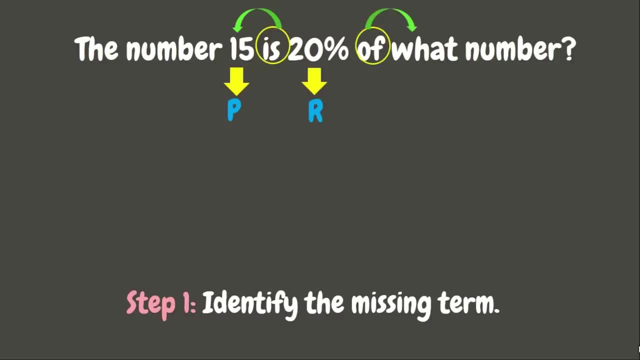 which comes after the word of is the base. This means that we are looking for the base. Now let's write the formula Again. let's use our triangle. Since we are looking for the base, this means that we need to divide percentage by the rate.